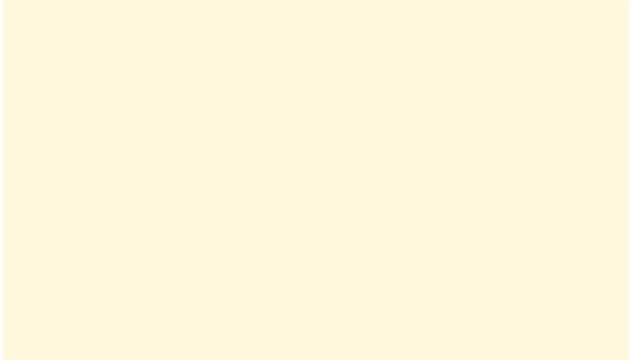 G'day. welcome to the TechMath channel. What we're going to be having a look at in this video is we're going to be having a look at how to solve some algebraic equations pretty instantly, okay. So, without much further ado, I'll show you the type of questions we'll be doing with these. We're going to be doing these types of questions where, say, we had something like 3x plus 5 and we're going to divide that whole lot by 7 and this is going to be equal to 2.. So we're going to be asked to solve a question like this. 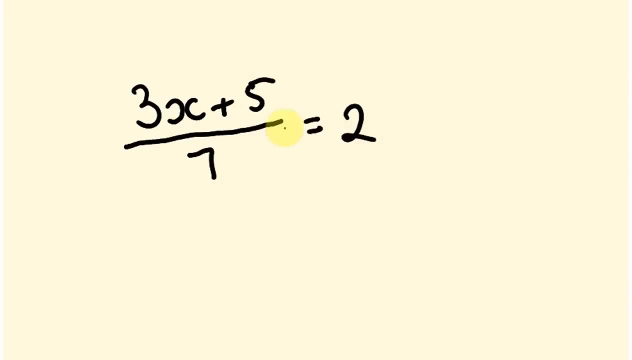 And they're not too hard, but you sort of there's a couple of things that are really really handy to know with them, and so you can solve them really, really quickly. So I'm going to show you a first step, one that you probably won't have to do after a while. you'll do it just in your head, straight away. 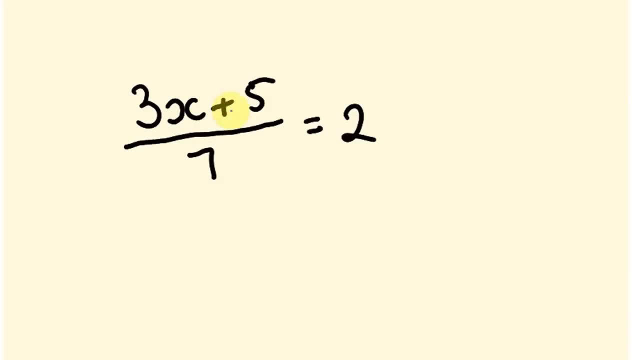 But first off, I think it's really important on this side to realise what's going on. So we're starting with an x and I'm going to be thinking about this in terms of bod mass and that sort of deal, like if we could actually do this. but I'm not going to be writing what we're going to be doing down here in terms of bod mass. I'm just going to be writing what we're going to be doing down here. 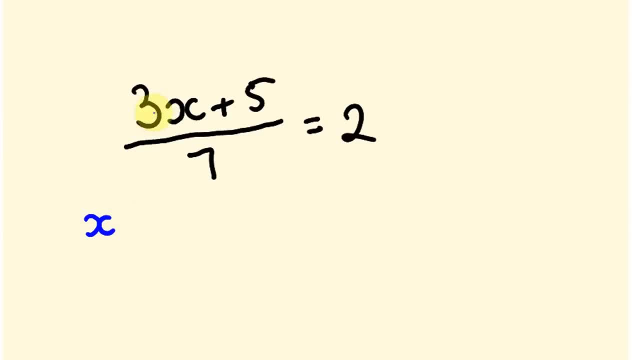 So we're going to be looking at x in terms of left to right, just in order of what's happening to it. So x first off, we're timesing it by 3, then we're adding 5 to it, and then we're getting this whole amount that we've got there and we're dividing it by 7 and we're getting the answer of 2.. 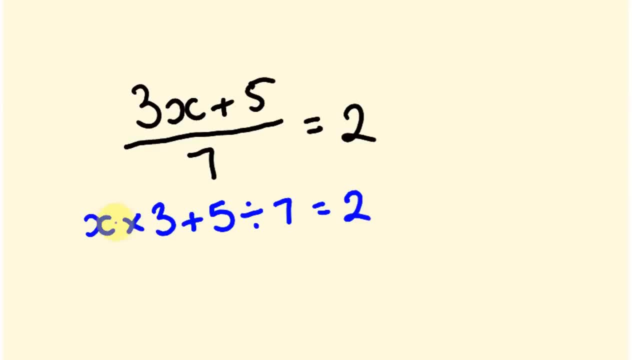 So, to get our answer, what we're going to do to find out what x is we're going to this time, we're running this way when we do it this time, but we're going to actually be running this way, And when we do this, we're going to be running in the reverse direction. 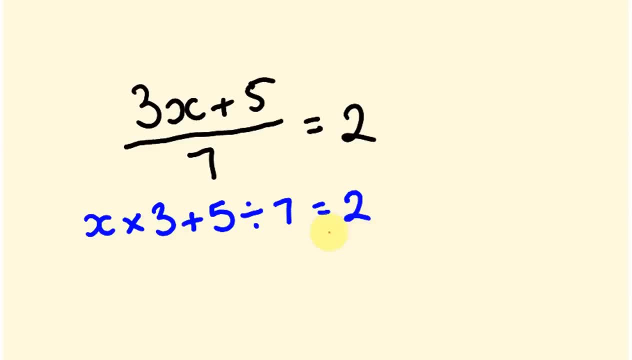 the opposite things. Okay, so we're going to start with 2, and, instead of dividing by 7, we're going to do the opposite, which is timesing by 7.. And then, instead of adding 5, we're going to take 5.. And then, instead of: 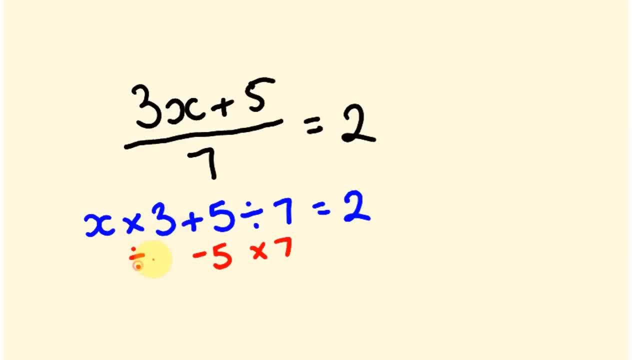 multiplying by 3, we're going to divide by 3.. Okay, so we'll be getting this direction. So 2 times 7 is 14.. Take away 5 is 9, divided by 3 is 3.. So x is equal to. 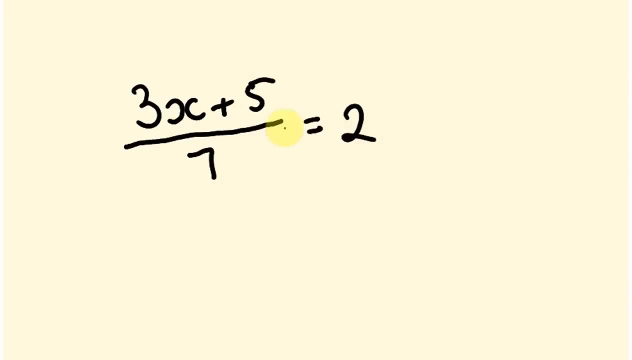 And they're not too hard, but you sort of there's a couple of things that are really really handy to know with them, and so you can solve them really, really quickly. So I'm going to show you a first step, one that you probably won't have to do after a while. you'll do it just in your head, straight away. 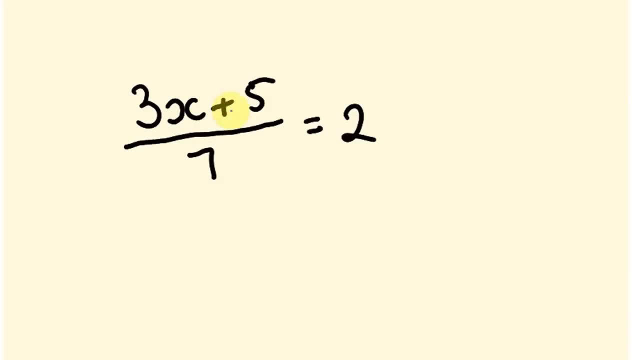 But first off, I think it's really important on this side to realise what's going on. So we're starting with an x and I'm going to be thinking about this in terms of bod mass and that sort of deal, like if we could actually do this. but I'm not going to be writing what we're going to be doing down here in terms of bod mass. I'm just going to be writing what we're going to be doing down here. 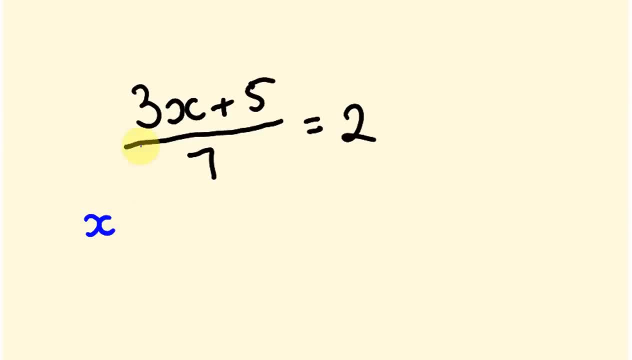 In terms of left to right, just in order of what's happening to it. So x, first off, we're timesing it by 3, then we're adding 5 to it, and then we're getting this whole amount that we've got there and we're dividing it by 7 and we're getting the answer of 2.. 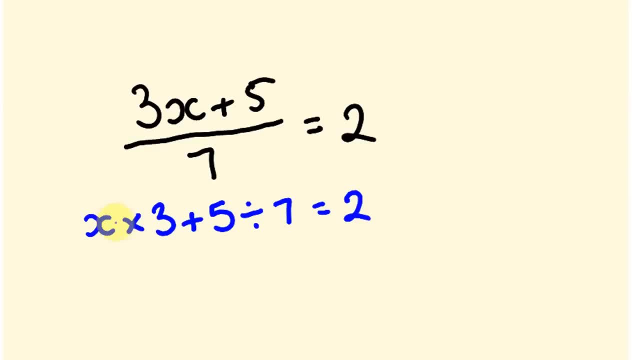 So, to get our answer, what we're going to do to find out what x is we're going to this time. we're running this way, while we do it this side, but we're going to actually be running this way And when we do this, we'll be running in a reverse direction. 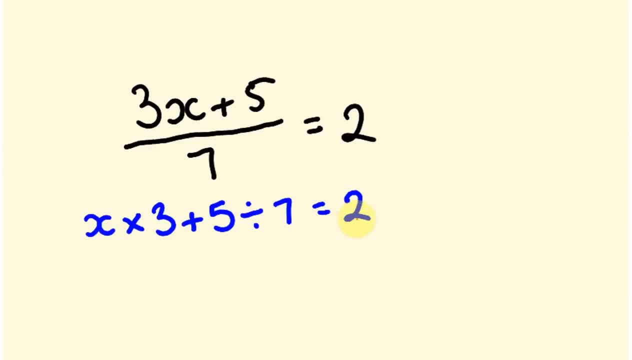 We're going to be doing the opposite things. Okay, so we're going to start with 2 and, instead of dividing by 7, we're going to do the opposite, which is timesing by 7.. And then, instead of adding 5,, we're going to take 5.. And then, instead of 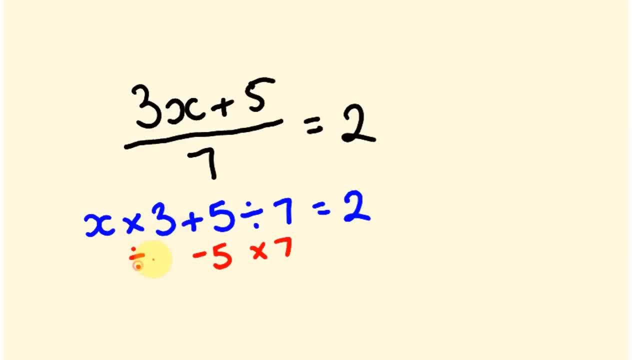 multiplying by 3, we're going to divide by 3.. Okay, so we'll be getting this direction. So 2 times 7 is 14.. Take away 5 is 9, divided by 3 is 3.. So x is equal to. 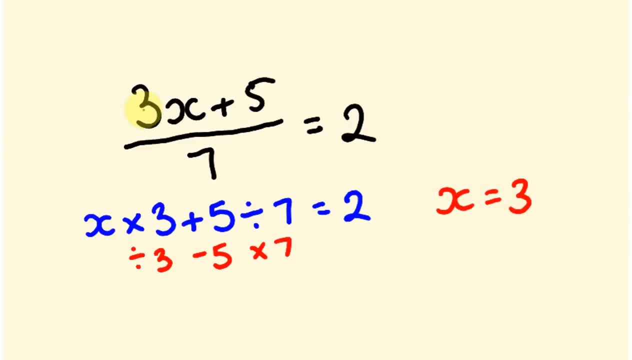 3. We can check this, because we can substitute this back into our equation here. So 3 times 3 is 9, plus 5 is 14, divided by 7 is 2.. So our answer is correct. Okay, do you see how we did that? So it's not overly. 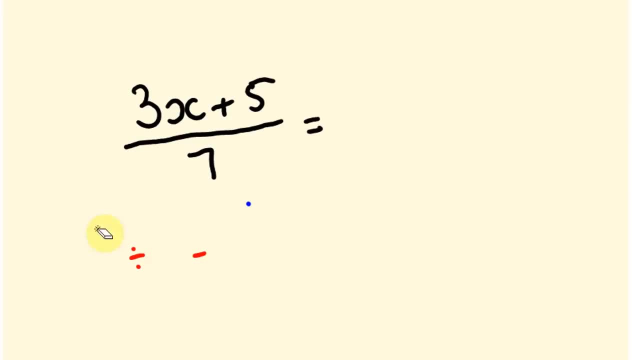 difficult. Some people do this, I think, quite naturally after they've been doing these types of equations, And so you hit this stage, you'll just be doing them anyway. So I'll give you another example of this. I'll give you an example like this one we just did, and then I'm going to give you. 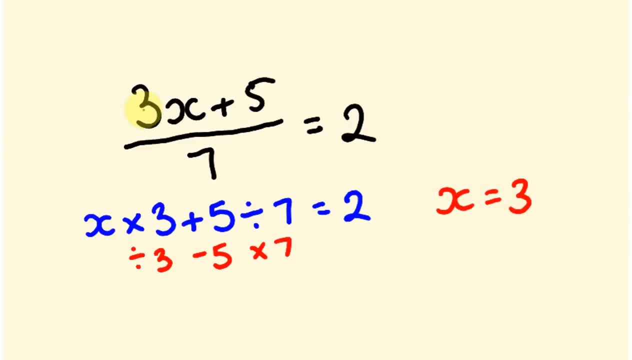 3. We can check this, because we can substitute this back into our equation here. So 3 times 3 is 9, plus 5 is 14, divided by 7 is 2.. So our answer is correct. Okay, do you see how we did that? So it's not overly. 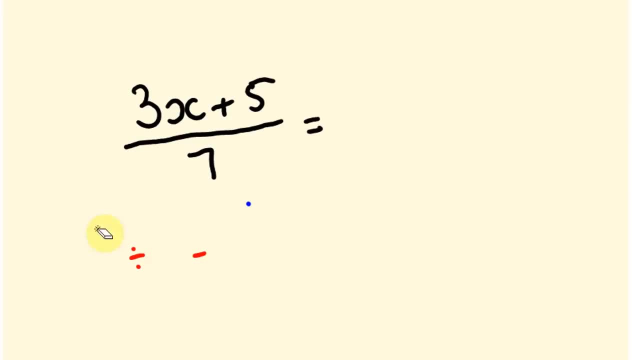 difficult. Some people do this, I think, quite naturally after they've been doing these types of equations. So you hit this stage, you'll just be doing them anyway. So I'll give you another example of this. I'll give you an example like this one we just did, and then I'm going to give you 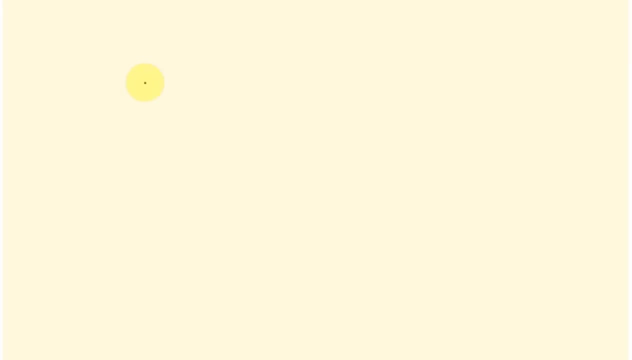 a few different types of examples. So say, I do a different one, Say we do 5x and from this we're going to take away what about? we take away 8, and I'm going to divide this by 3 and the answer is 4.. Okay, 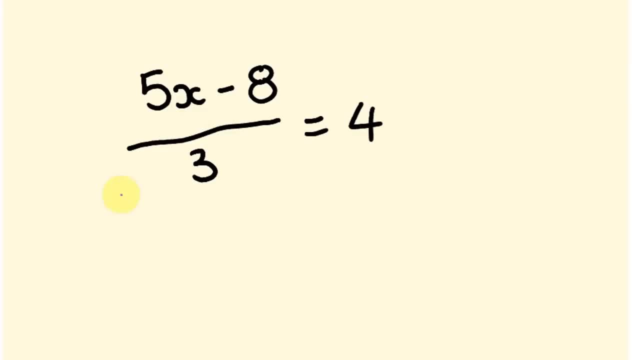 So if we were doing this again, we could write out the order we were doing this. We're getting 5,. well, first off, we're getting x here and I'll write that out with x, and we're timesing it by 5,. 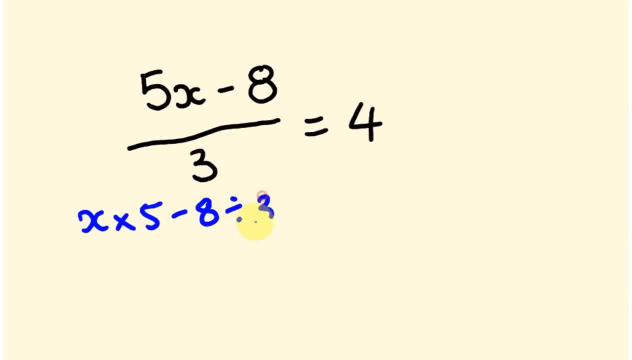 we're taking away 8, we're dividing that answer by 3.. Okay, we're going this times this: we're taking away 8, and then we're dividing this whole bit by 3 here. Then we're getting this answer of 4.. 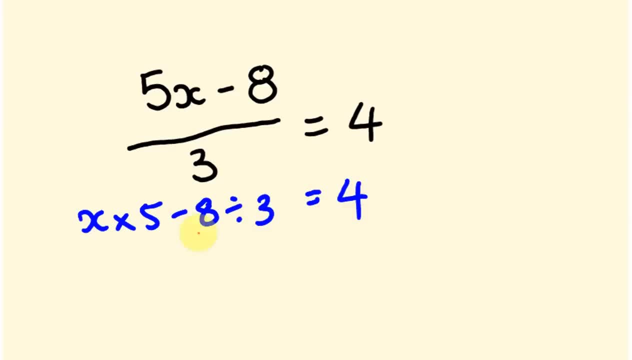 So what we're going to do is we're going to do the opposite here. We're going to run in this direction. instead, we're going to times by 3, add 8, divide by 5 to get our answer. Okay. so 4 times 3. 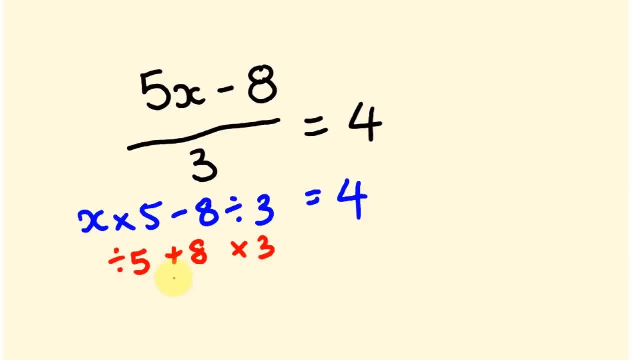 is 12, plus 8 is 20, divided by 5. our answer is: 20 divided by 5 is 4.. So x is equal to 4.. And we can substitute this in. to check it once again: 5 times 4 is 20. 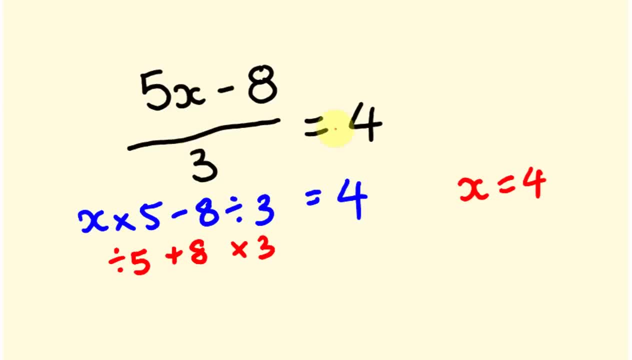 take away: 8 is 12, divided by 3 is 4.. No problem, So what about we do a couple of different ones of these? Okay, so this really relies upon you knowing the order of operations at bod mass ped massing, which is something you should know anyway. 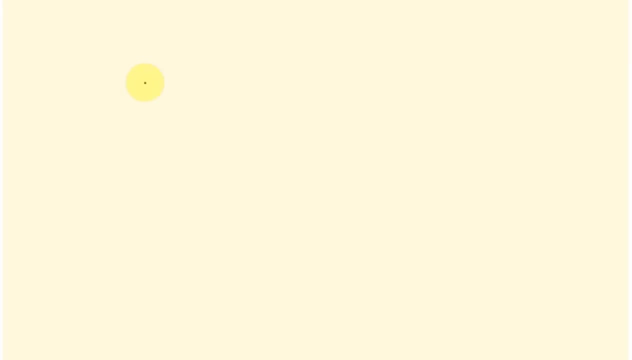 a few different types of examples. So say, I do a different one, Say we do 5x and from this we're going to take away what about? we take away 8, and I'm going to divide this by 3 and the answer is 4.. Okay, 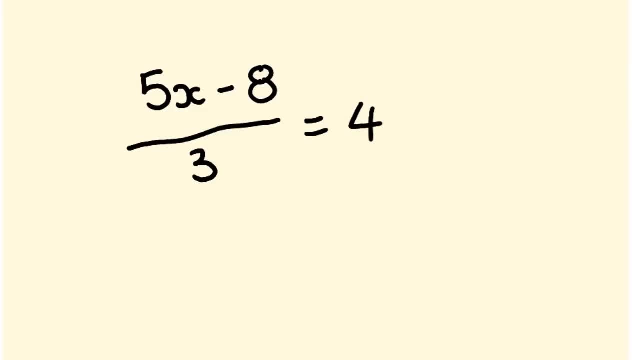 So if we were doing this again, we could write out the order we were doing this. We're getting 5, well, first off, we're getting x here. I'll write that out with x and we're timesing it by 5,. 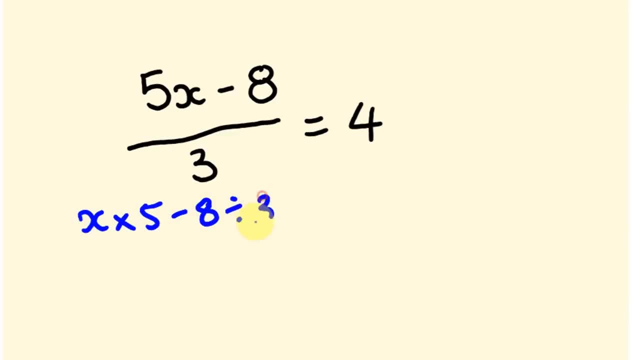 we're taking away 8, we're dividing that answer by 3.. Okay, we're going this times this: we're taking away 8, and then we're dividing this whole bit by 3 here. Then we're getting this answer of 4.. 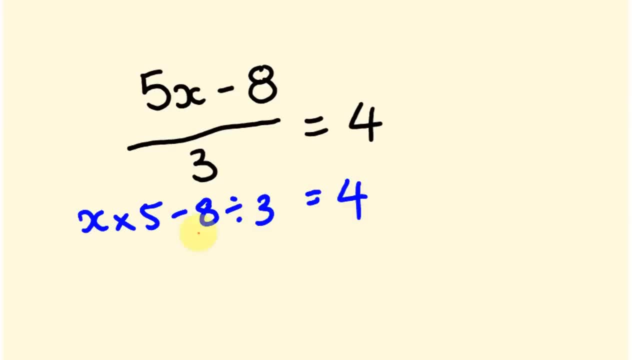 So what we're going to do is we're going to do the opposite here. We're going to run in this direction. instead, we're going to: times by 3, add 8, divide by 5 to get our answer Okay. so 4 times 3 is 12,. 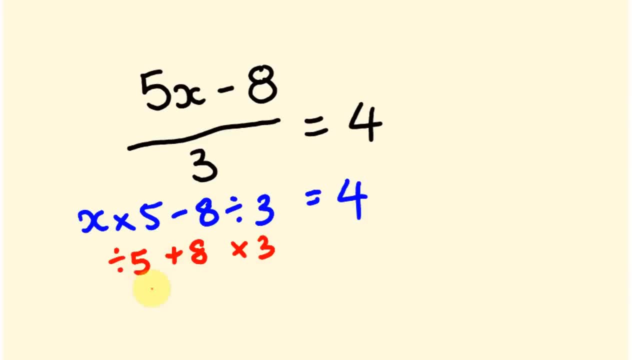 plus 8 is 20, divided by 5,. our answer is: 20 divided by 5 is 4.. So x is equal to 4.. And we can substitute this in. to check it once again: 5 times 4 is 20, take away 8. 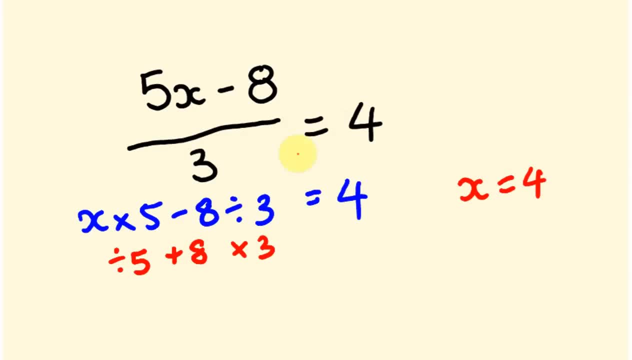 is 12.. 5 times 3 is 4.. No problem, So what about we do a couple of different ones of these? Okay, so this really relies upon you knowing the order of operations at BodMass- PedMass, which is something you should know anyway. if you're doing these, you have to. 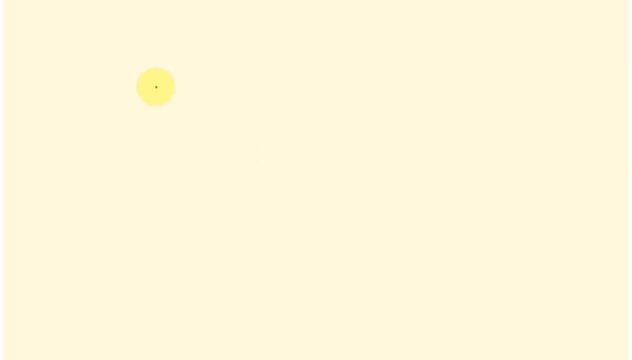 know it. Okay. so the next one I'm going to do is say this one: What about we do x squared and we add 7 to that, and we've got the square root of that, and we're going to add 5, and the answer equals 9.. 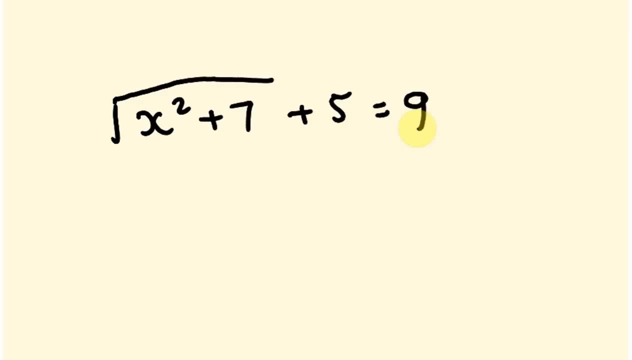 Okay, Alright, Okay, so first off, work out which order we're doing these in. Okay, so we're going first off. we're getting x. okay, Then what we're doing to x is: it's being squared, so it's being times by itself. I'm just going to do a little. 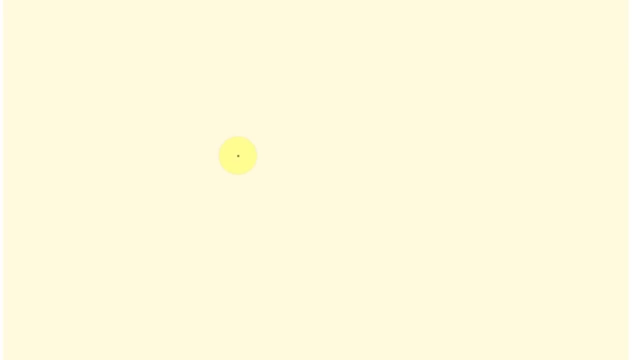 if you're doing these, you have to know it. Okay, so the next one I'm going to do is say this one: What about we do x squared and we add 7 to that and we've got the square root of that and we're going to. 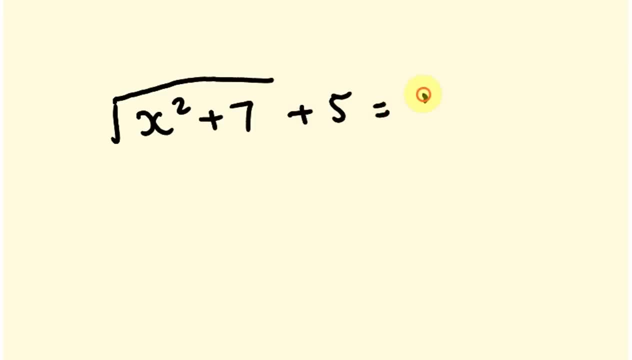 add 5. And the answer equals 9.. Okay, Alright. Okay, so first off, work out which order we're doing these in. Okay, so we're going first off. we're getting x. Okay, Then what we're doing to x is it's being: 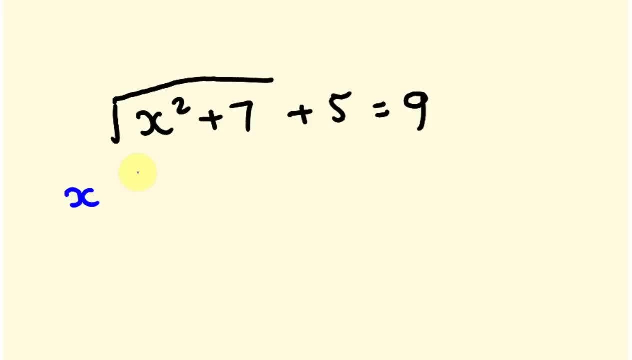 squared, so it's being times by itself. I'm just going to do a little squared here, Okay? Then we're adding 7, we're square rooting the answer, and then we're adding 5.. Then we're adding 7, we're square rooting the answer, and then we're adding 5.. 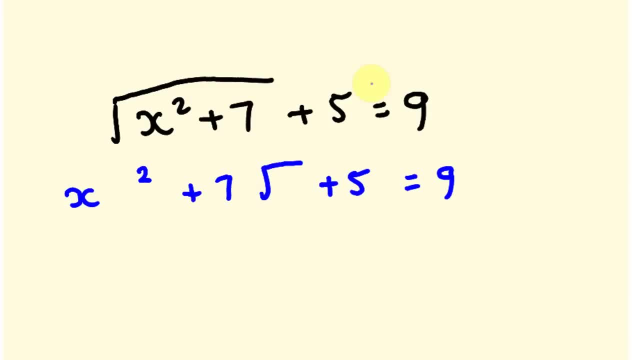 And we're getting this answer of 9.. Notice, I haven't tried to write it in any formula up here. I'm just trying to write what's happening here, because we're going to be doing the opposite. Okay, I think that's a really great idea to be able to do. 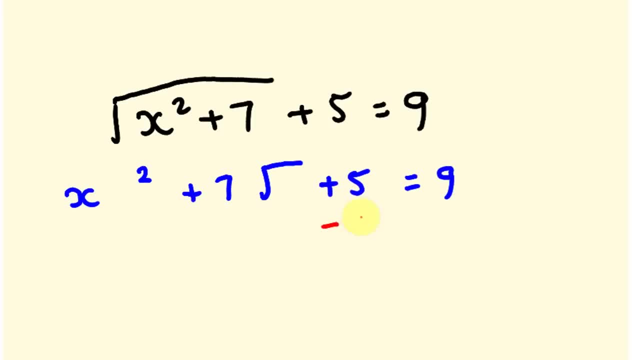 So what we're going to do is we're going to start with our 9, we're going to now do the opposite. We're going to take 5, we're going to the opposite of square. root is squared, so we're going to square. 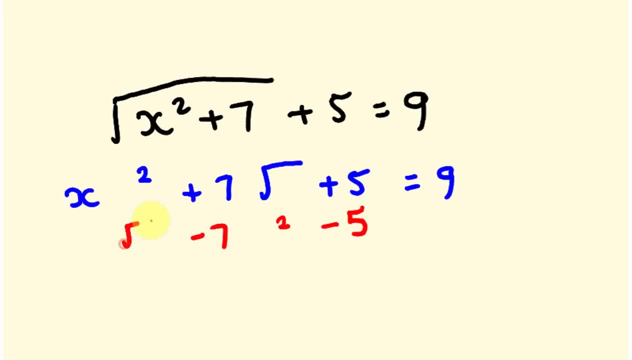 We're going to subtract 7, then we're going to square root our answer And we're going to get our answer here. so 9 take away 5 is 4.. 4 squared 4 times 4 is 16.. 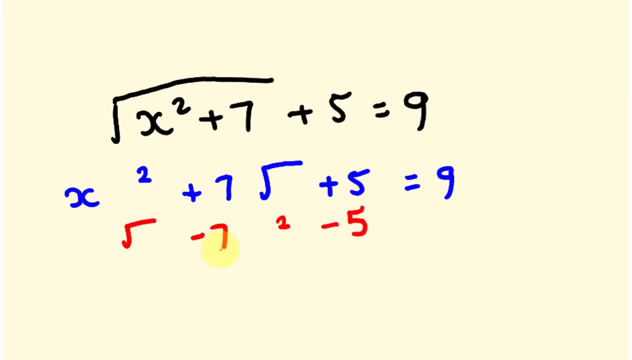 16. take away 7 is 9.. The square root of 9 is 3.. So x equals 3.. Now let's check that out. So let's just substitute this in x: squared 3 times 3 is 9, plus 7 is 16.. 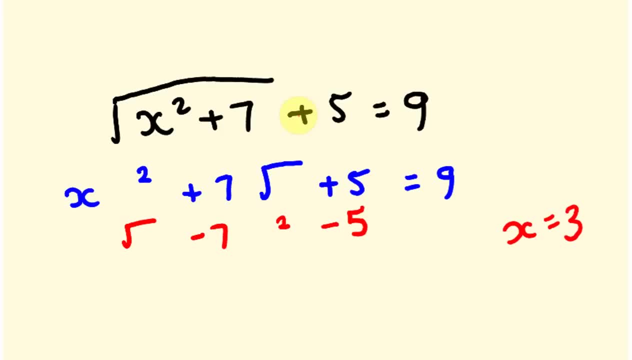 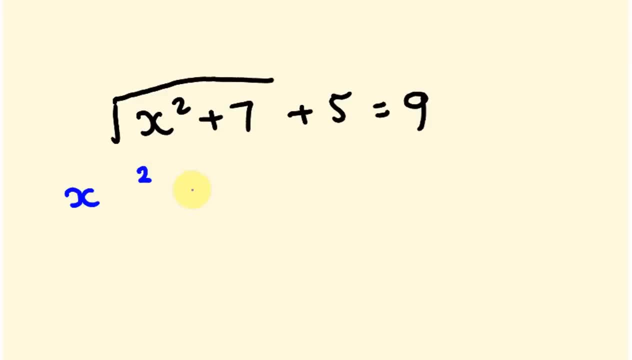 squared here, okay, Then we're adding 7, we're square rooting, and then we're adding 5, and we're getting this answer of 9.. Notice, I haven't tried to write it in any formula up here. I'm just trying to write what's happening here. 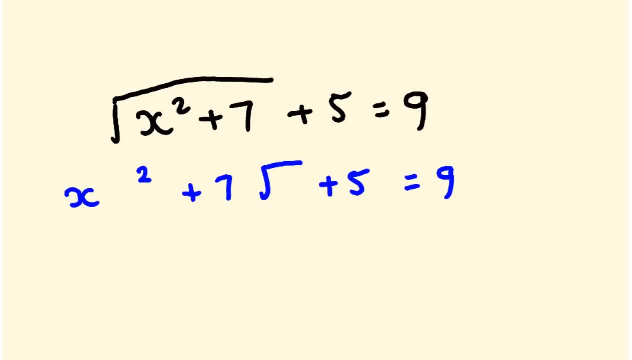 because we're going to be doing the opposite. okay, I think that's a really great idea to be able to do. So what we're going to do is we're going to start with our 9, we're going to now do the opposite. We're going to take 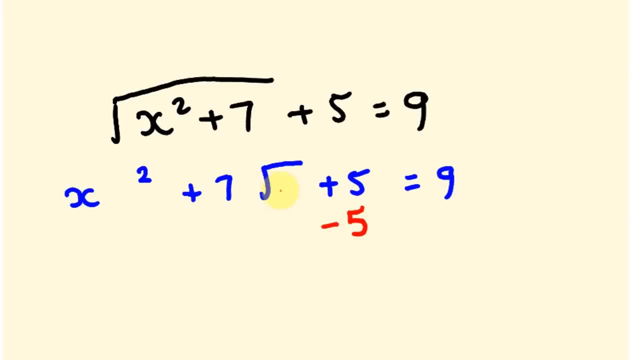 5,. we're going to the opposite of square. root is squared, so we're going to square. we're going to subtract 7, then we're going to square root- our answer- and we're going to get our answer here. so 9,. 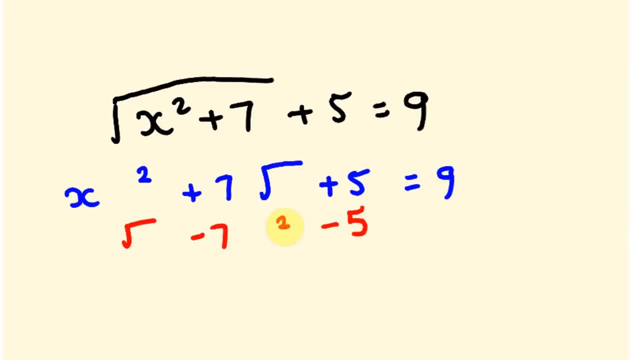 take away: 5 is 4,. 4 squared 4 times 4 is 16, 16,. take away: 7 is 9,. the square root of 9 is 3, so x equals 3.. Now let's check that out. so let's just substitute this in: x squared 3 times. 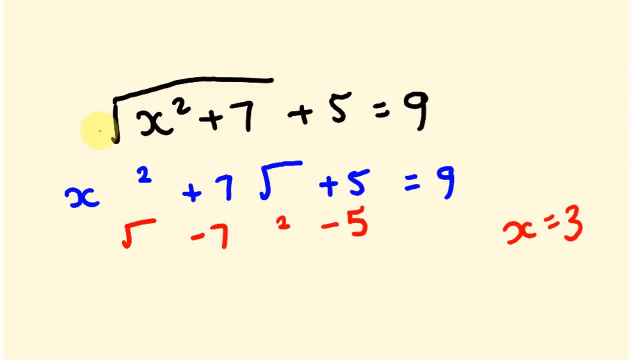 3 is 9, plus 7 is 16,. the square root of 16 is 4, plus 5 equals 9.. Our answer is correct. Alright, a couple more examples here. Hopefully you're doing well on these and hopefully this is something you looked at and go. 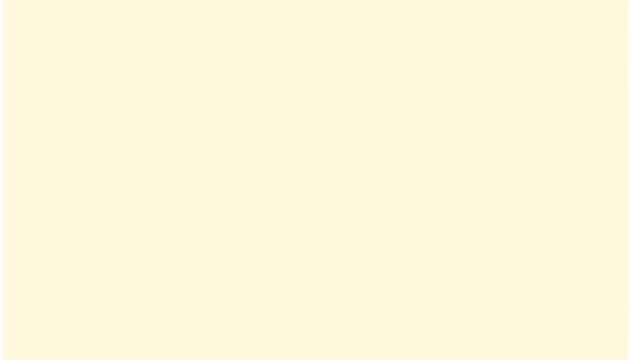 hey look, I already do this because that's fairly possible as well. Okay, what about we do this one? What about we get 2x, the square root of 2x, and we're going to put that over 2, and we're going to make that equal 2.. 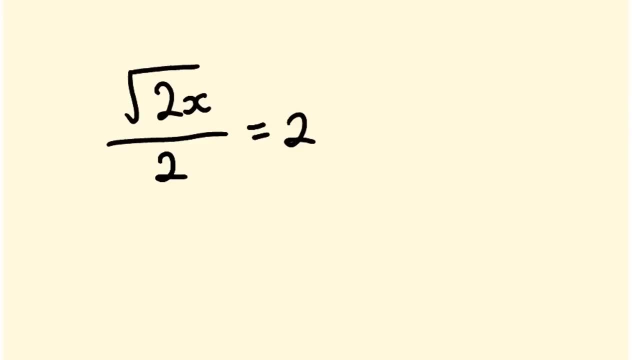 Okay, so first off, we have to work out what order everything's happening in here. so what we did is we're starting with x and that's being times by 2, and then what's happening is that whole amount's being square rooted. okay, so, square root, and then this whole answer here. 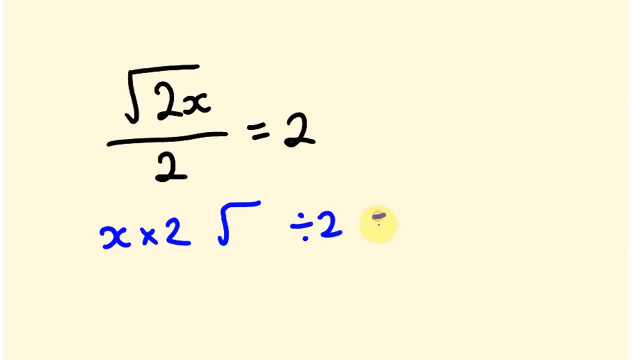 is being divided by 2,, so divided by 2, and this is equally 2.. So now let's do the opposite, okay. so divide by 2, the opposite is times by 2, the opposite of square root is to square, the opposite of 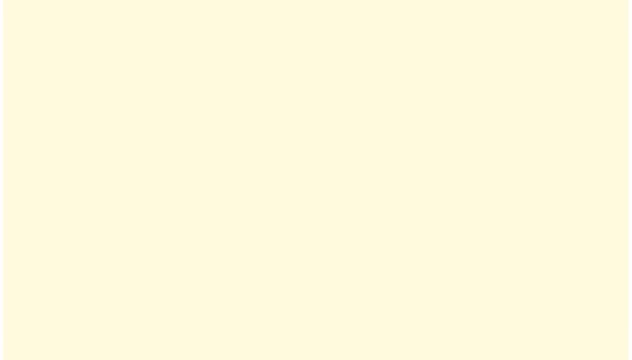 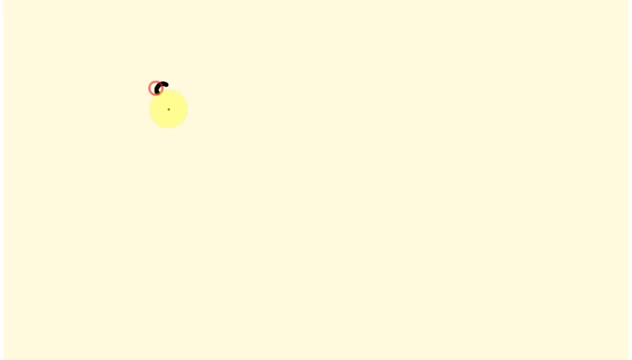 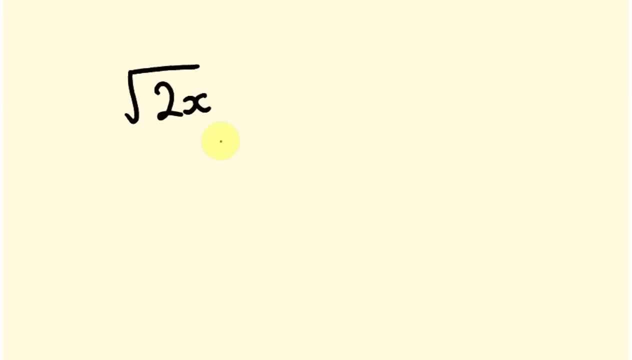 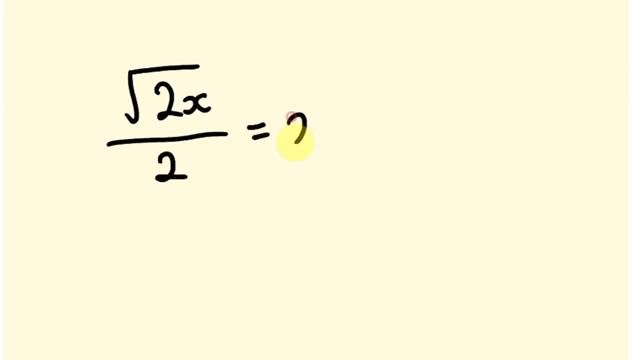 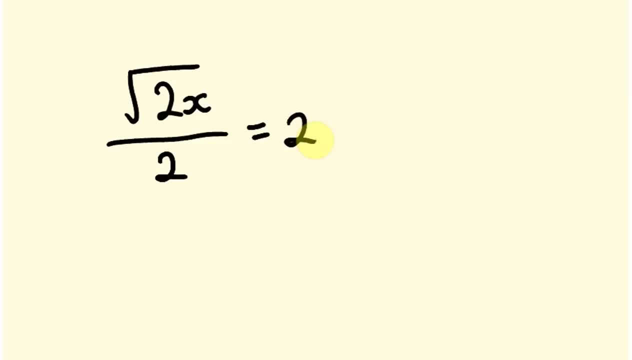 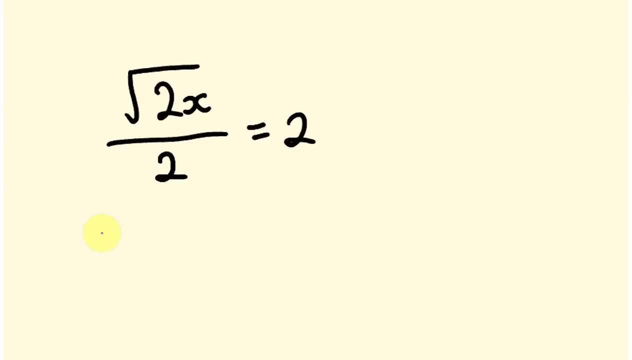 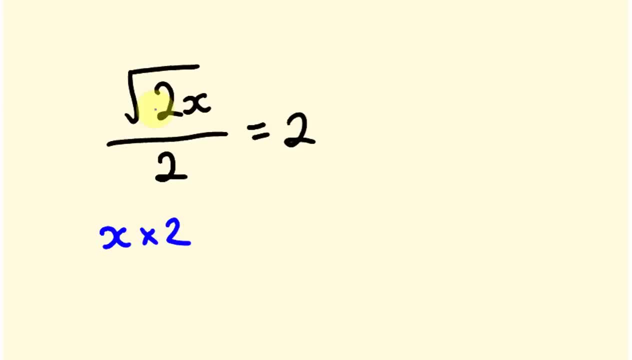 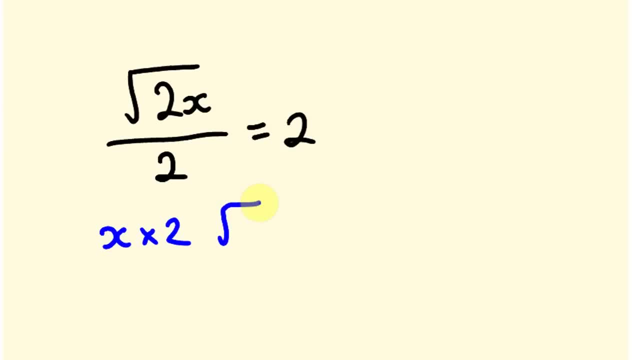 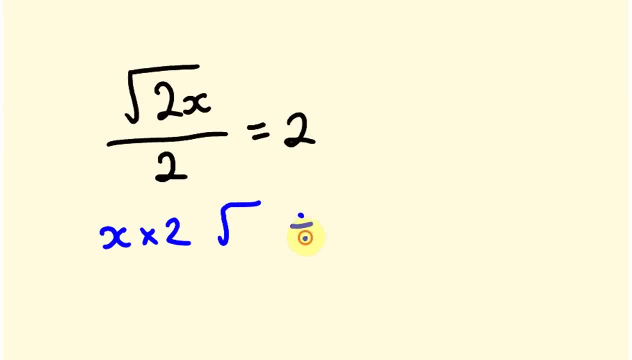 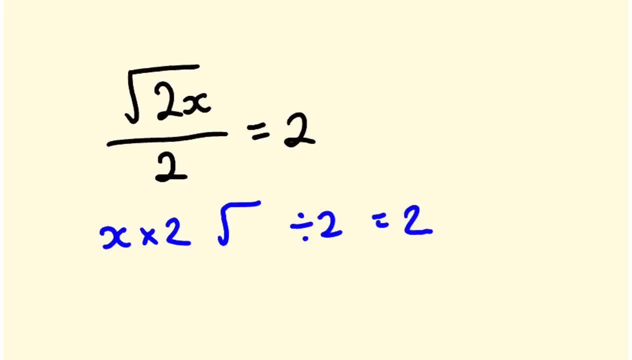 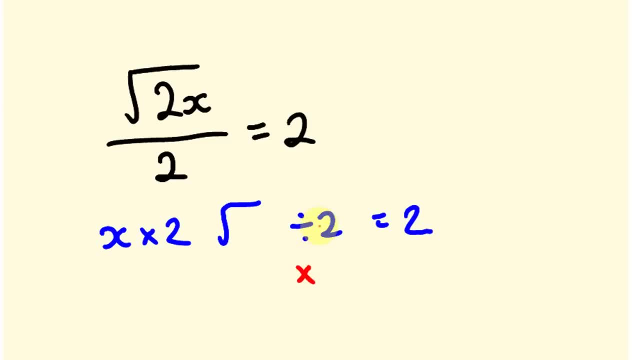 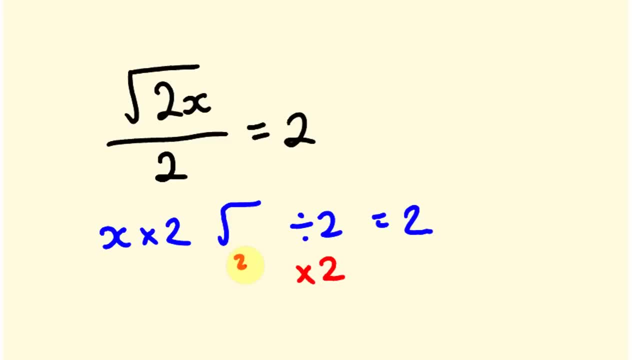 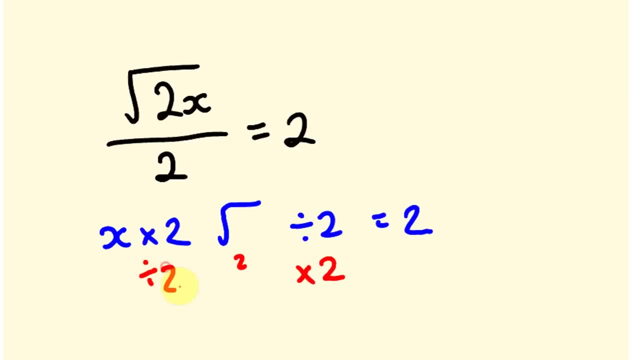 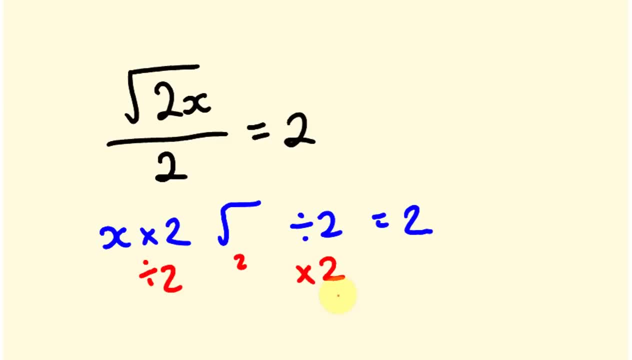 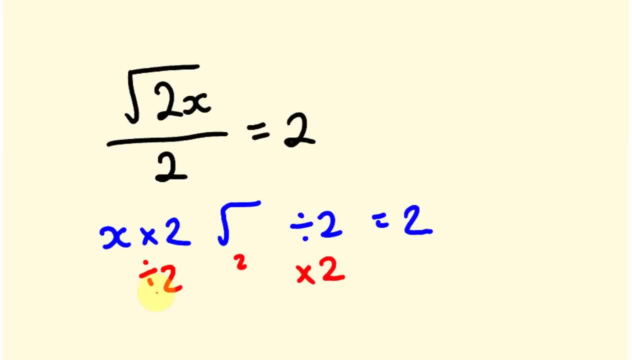 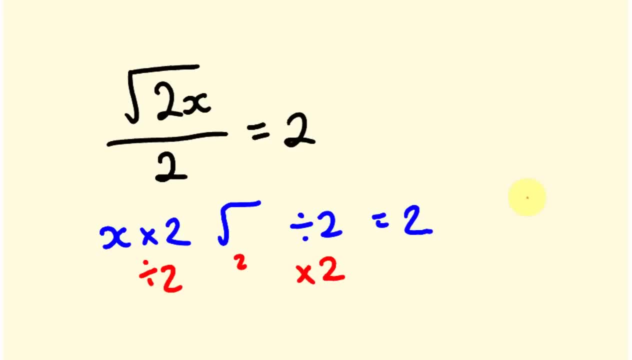 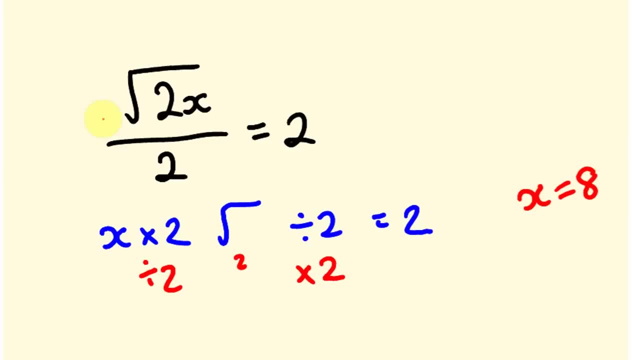 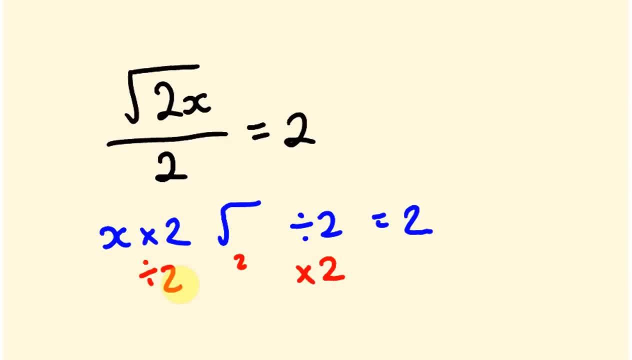 timesing by 2 is to divide by 2, it's a lot of 2's, Okay. so 2 times 2, is 4, 4 squared is 16,. 16 divided by 2 equals 8.. 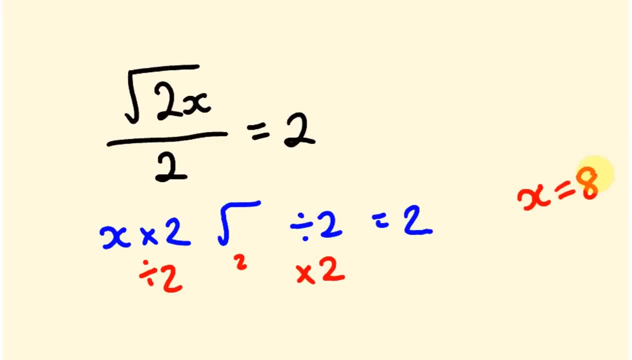 Okay, so x equals 8.. Let's substitute in our answer- it's a really good thing to do so- 2 times 8 is 16, the square root of 16 is 4, 4 divided by 2 is 2.. Our answer: 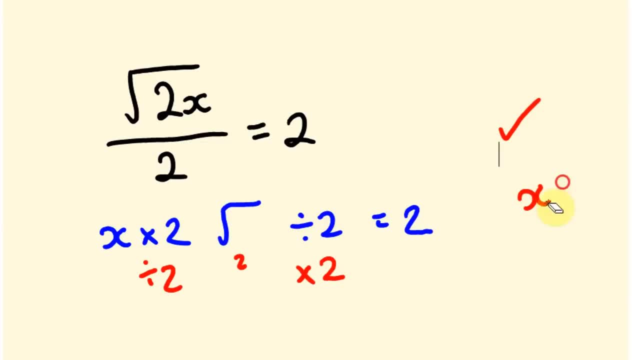 is correct. One lucky last example here: okay, So let's get rid of those. And okay, our last example here is: say what we do is we go. what about 5x minus 5x minus 6, okay, and then we're going to. 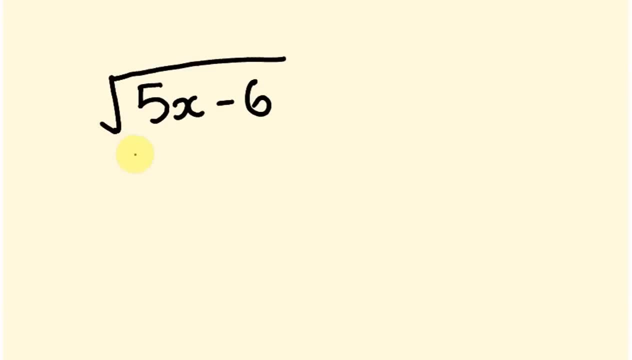 get that and we're going to square root that, okay, and then what we're going to do is times it by 4, and divide it by 2, okay, I wonder what that's going to equal. that will equal 6.. 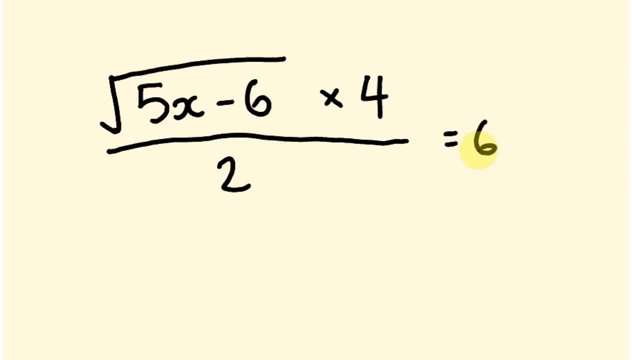 Okay, so let's see if we can work this one out. This is a big one, yeah, Okay, Alright, so let's do this 5x. this is like: first we're getting 5, x, we're timesing it by 5,. 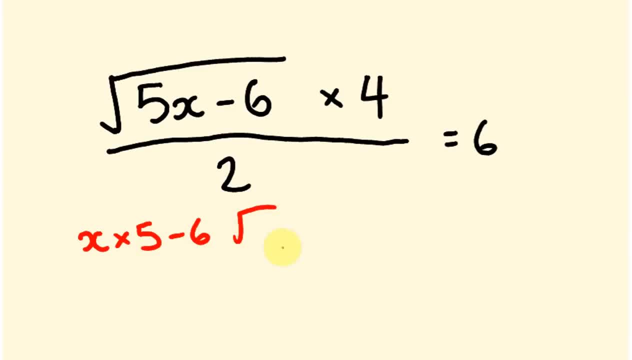 we're subtracting 6,, we're square rooting it, we're timesing that by 4, and then we're dividing by 2, and this equals 6.. Okay, so let's see if we can do this. Let's do the opposite here. so we're going to times by 2,. 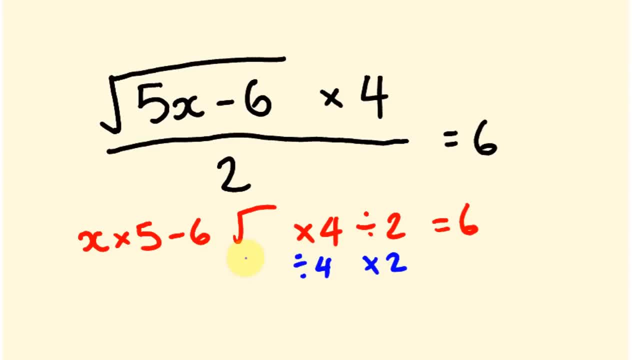 we're going to divide by 4,. we're going to the opposite of the square: root is squared. we're going to add 6, we're going to divide by 5,. okay, in that order. So 6 times 2 is 12, divided by 4 is 3, 3 squared is 9, 9 plus 6 is 15,, 15 divided by 5.. 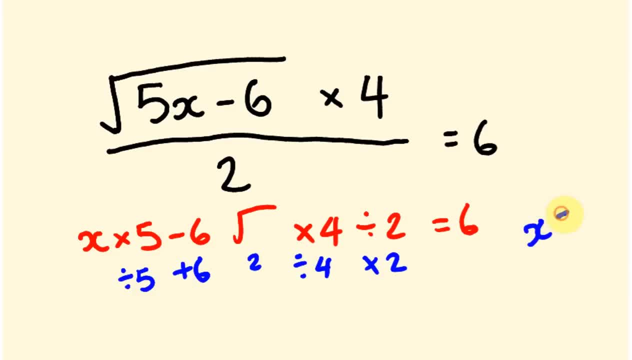 Okay, so x equals 3.. Alright, so let's just substitute that: in 5 times 3 is 15,. take away: 6 is 9,. the square root of 9 is 3,. 3 times 4 is 12,. 12 divided by 2 is 6.. 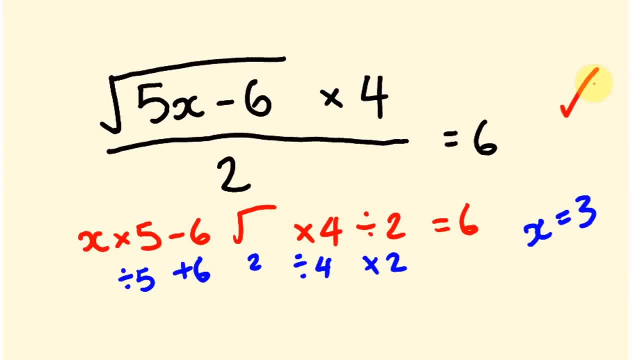 So our answer is correct. I was a bit worried about that one, I must say. I was making that one off the top of my head, so we didn't do it too badly. I was expecting it to be good, but there you go. Anyway, hopefully that was a. 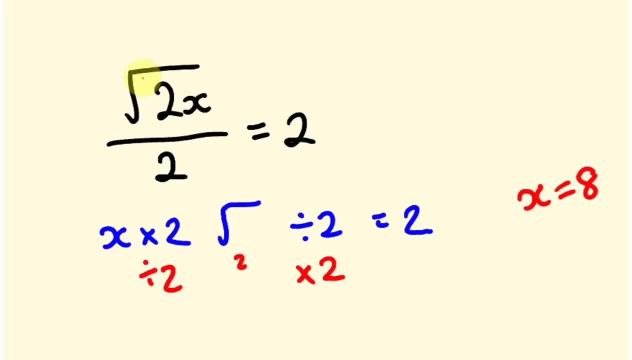 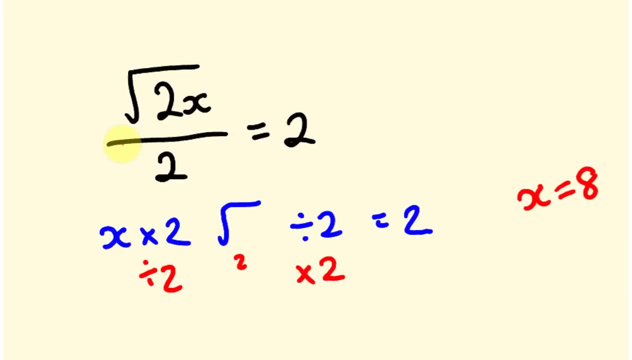 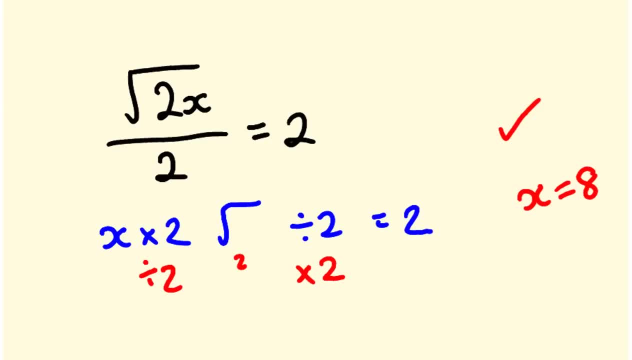 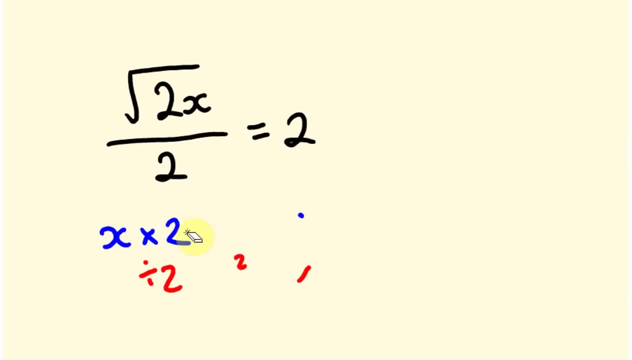 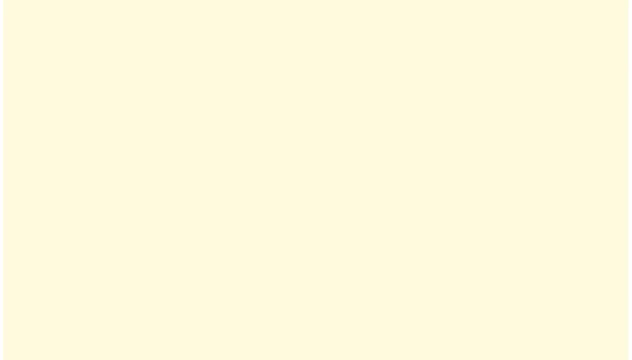 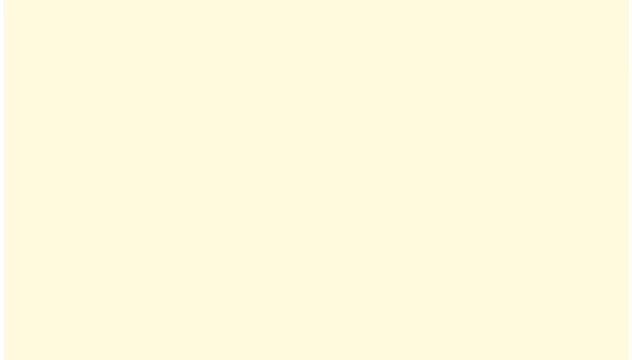 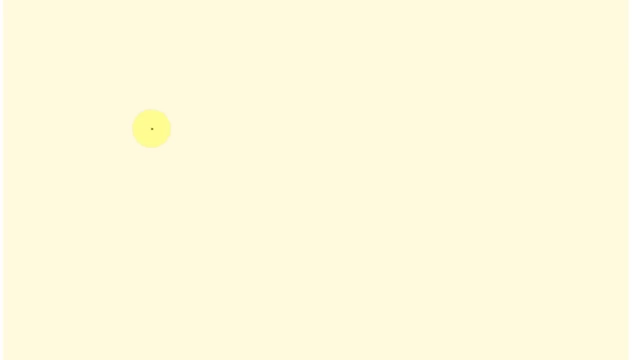 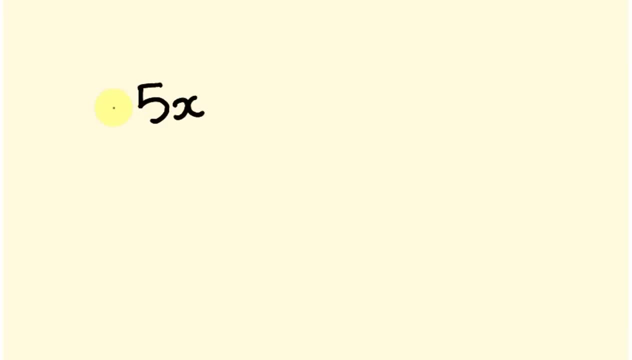 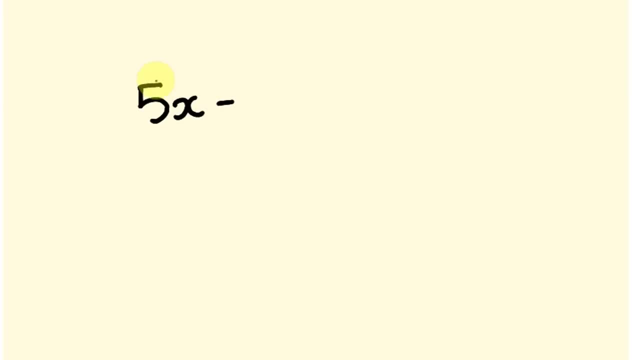 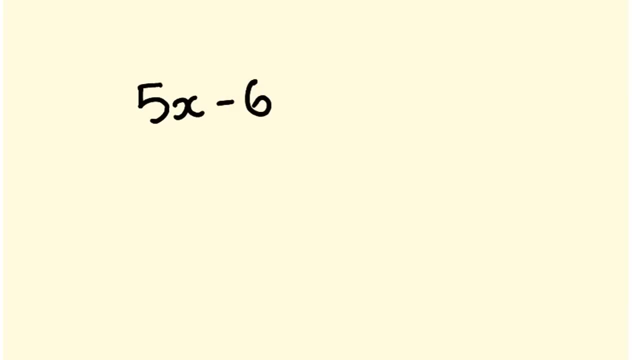 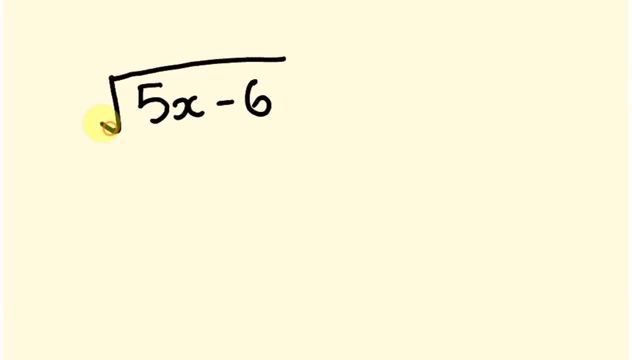 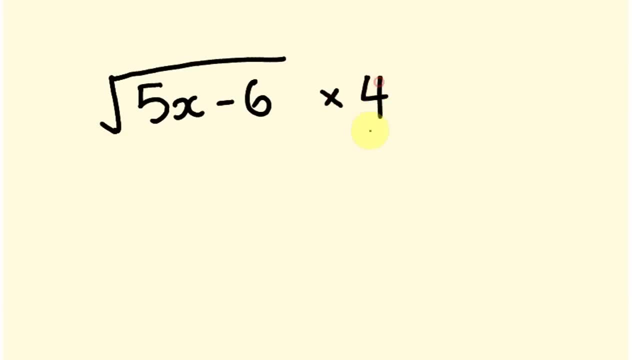 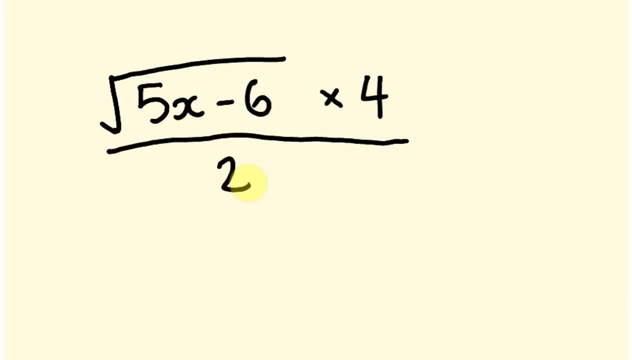 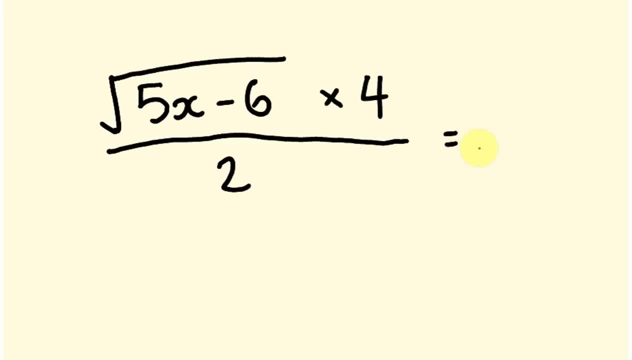 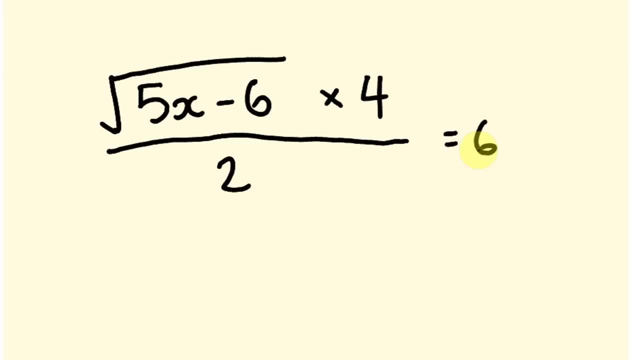 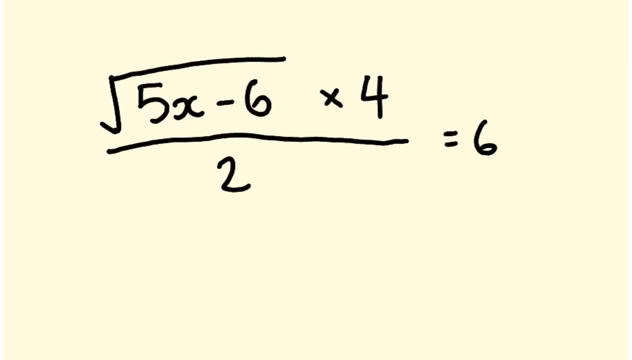 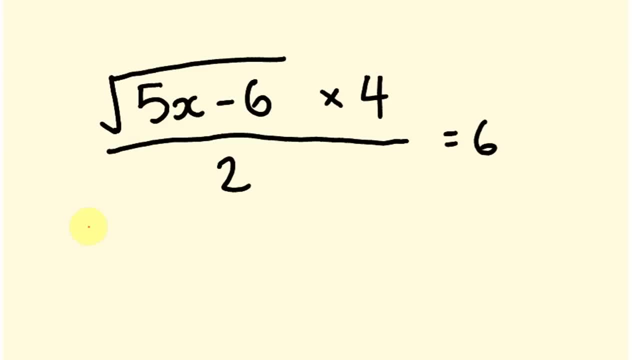 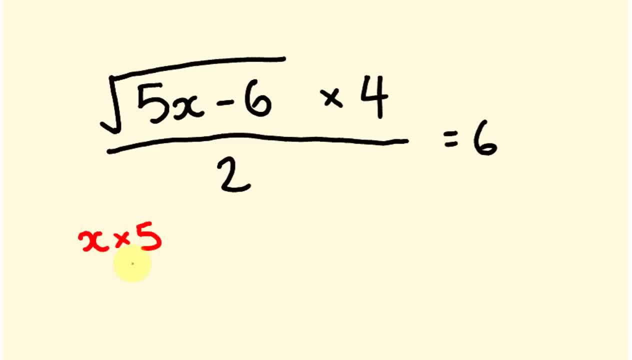 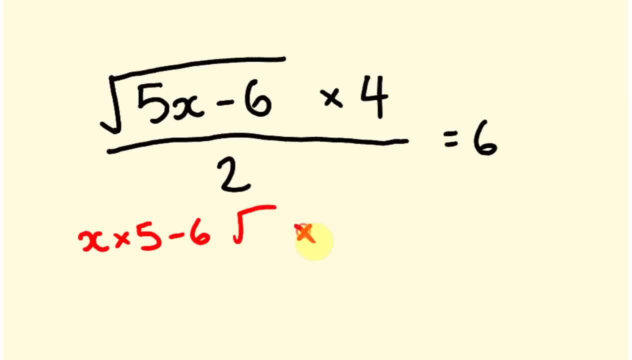 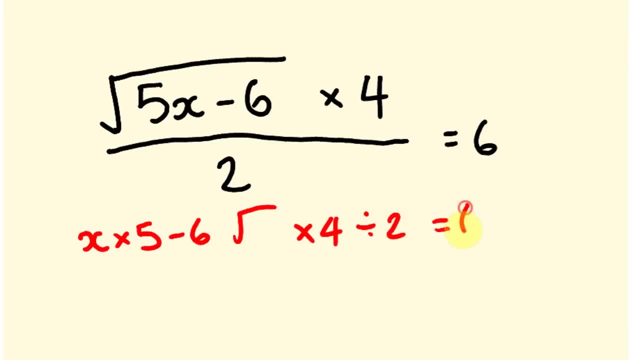 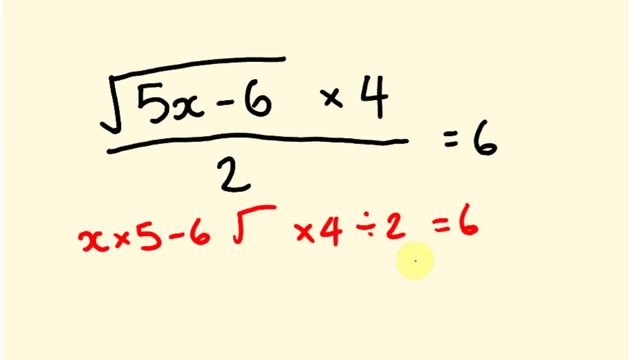 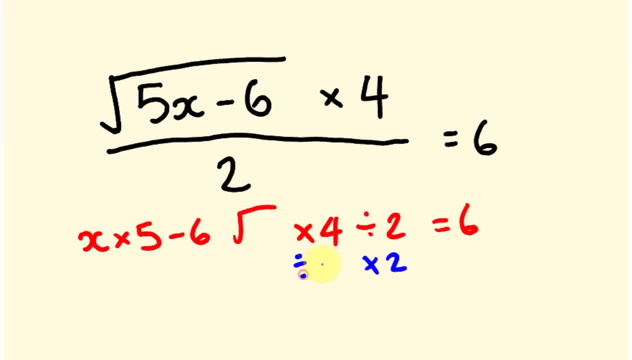 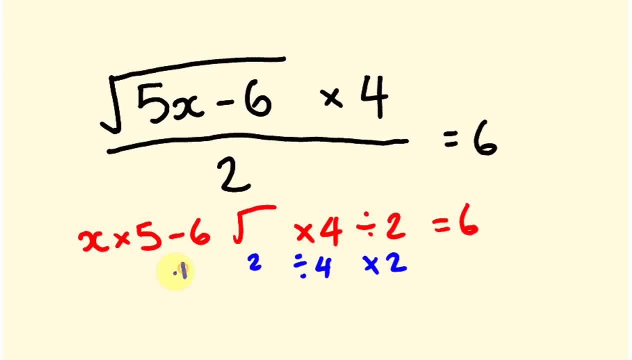 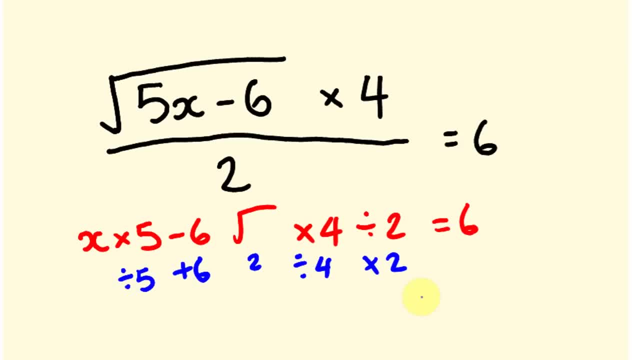 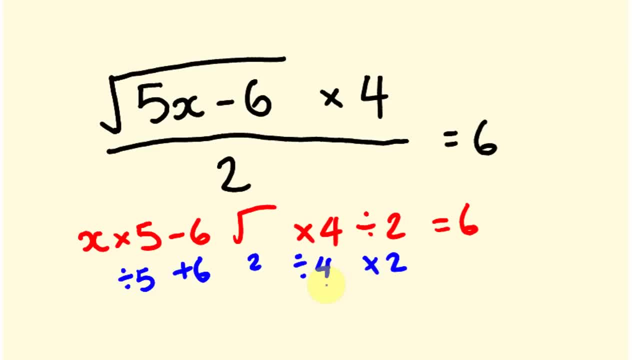 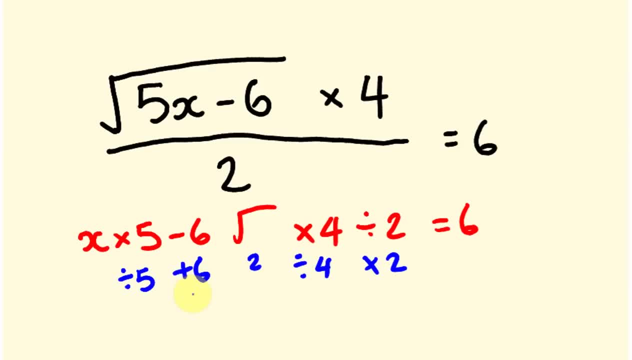 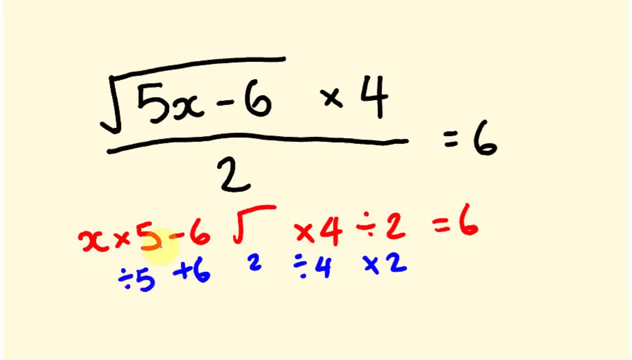 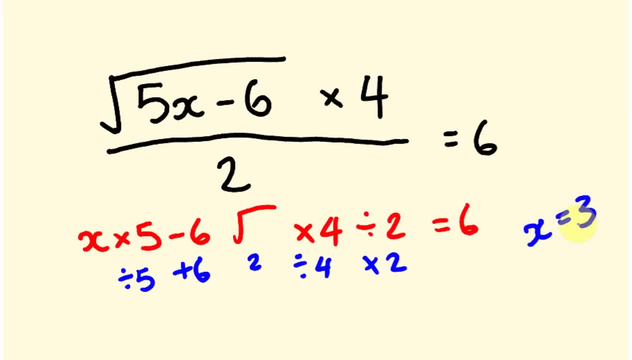 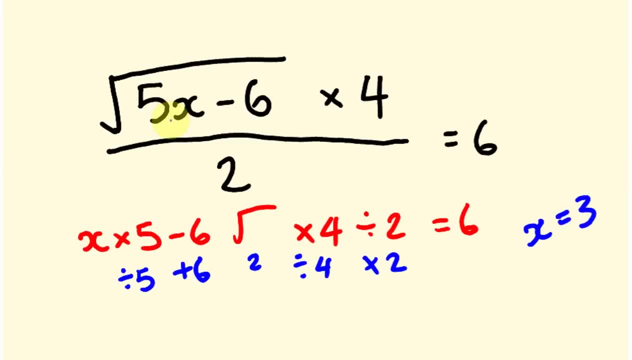 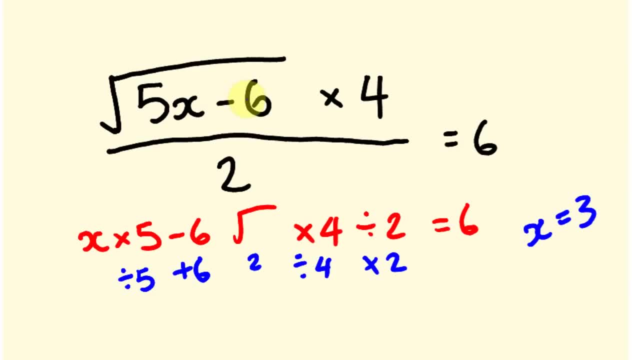 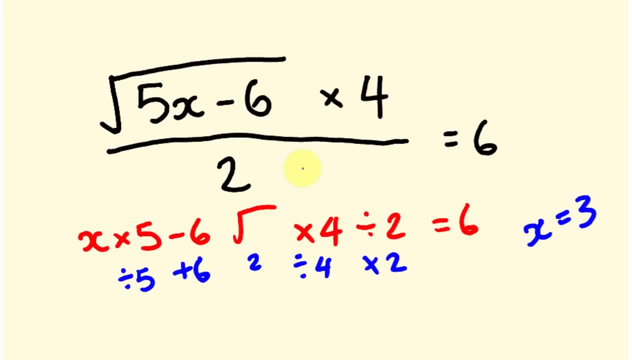 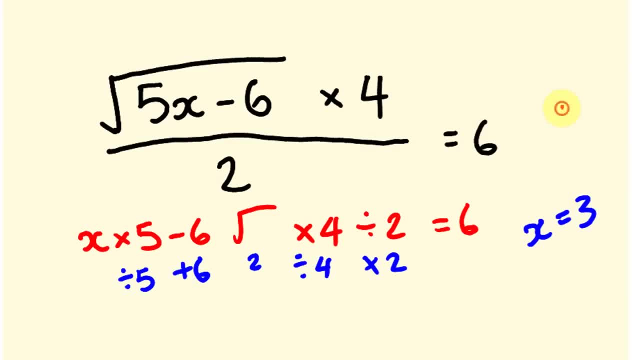 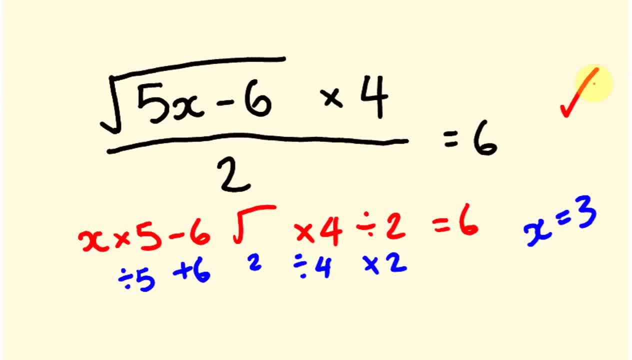 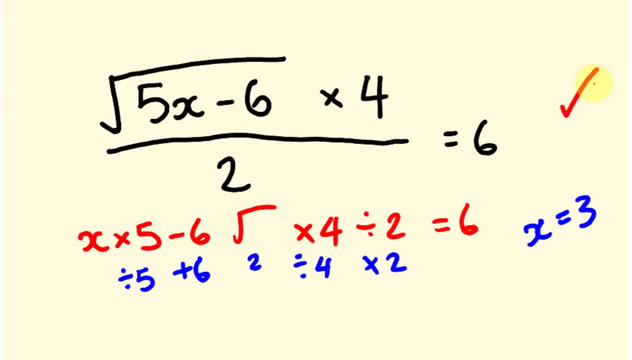